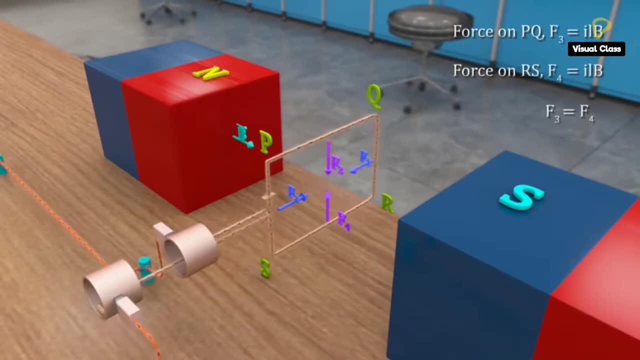 the same for both forces. the magnetic force F1 and F2 are equal in magnitude and have the same solution for both forces. The effect of the force F1 on SP and on QR is same in direction and have the same line of action. 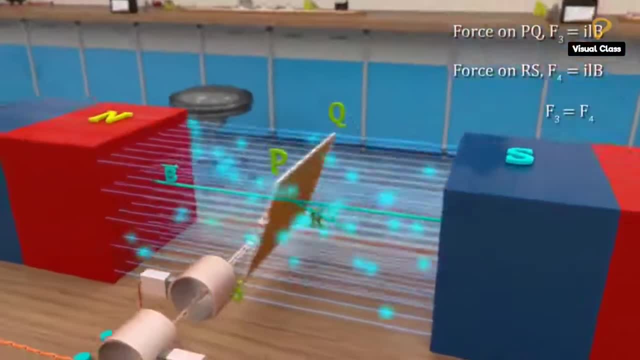 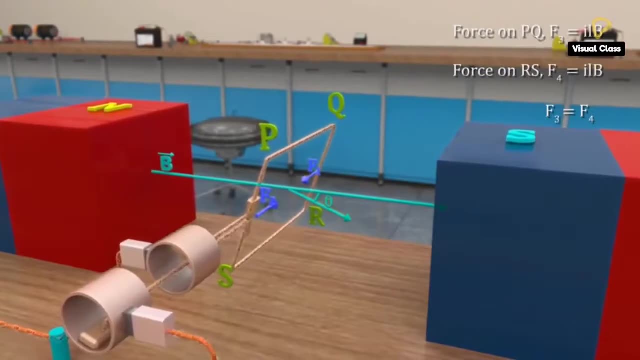 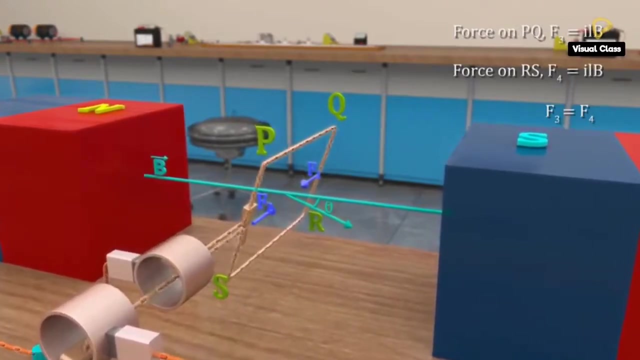 Let the loops normal, make an angle theta with the magnetic field. Forces on SP and QR are equal and opposite to each other and they have the same line of action. Hence they produce a net force equal to 0 and net torque also equal to zero. Magnitude of the force on PQ is equal to 0. 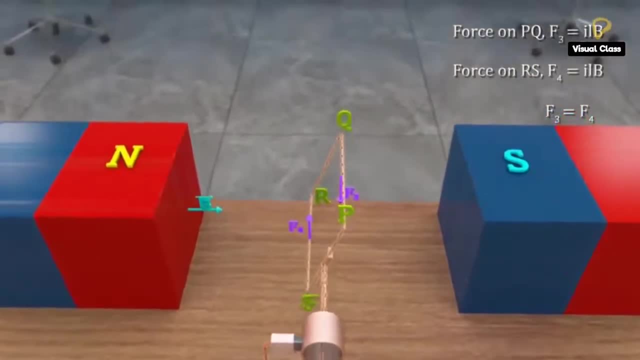 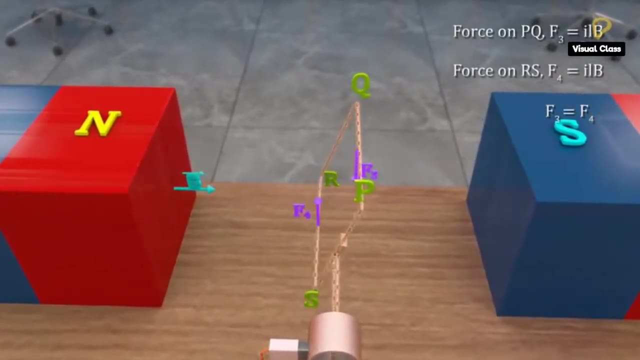 Magnitude of the force on PQ is equal to 0 and net torque is also equal to 0.- equal to the magnitude of force on RS. but they don't have the same line of action, Hence they produce a couple, due to which the coil tends to rotate in the clockwise direction. 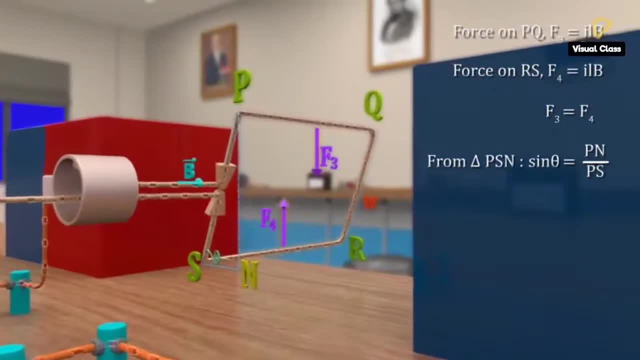 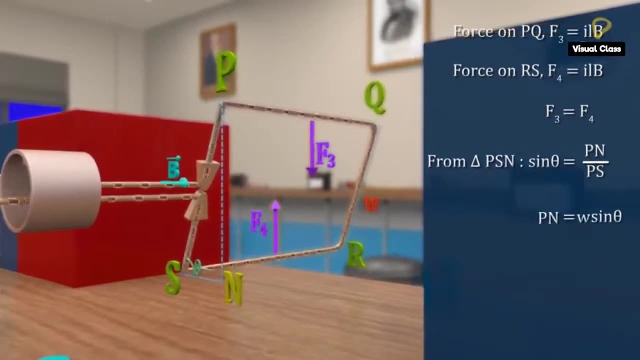 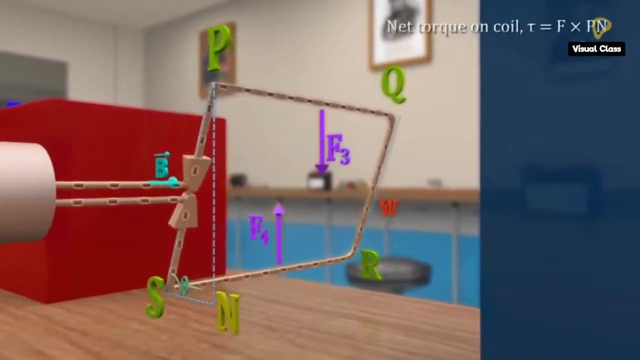 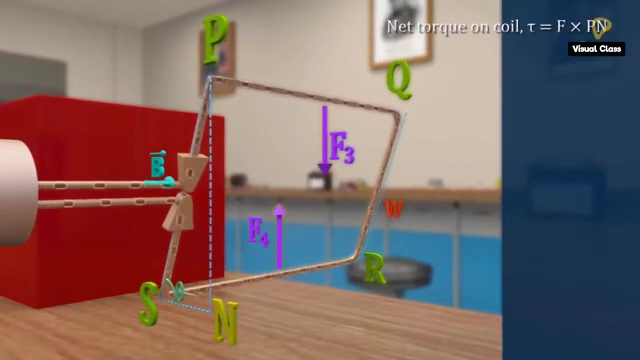 From triangle. PSN sine theta is equal to PN by PS. This gives the distance between the forces PN equal to W sine theta. Net torque acting on the coil is equal to the product of magnitude of force and the perpendicular distance between the forces WL is equal to area of the. 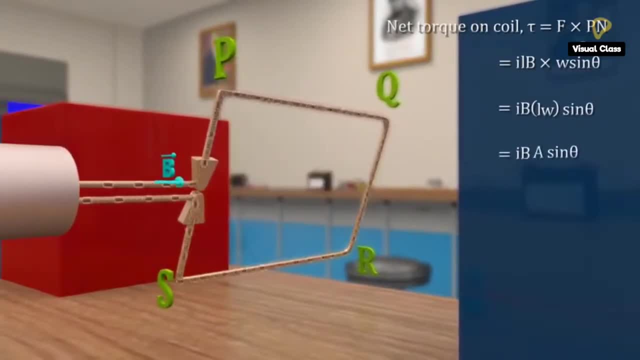 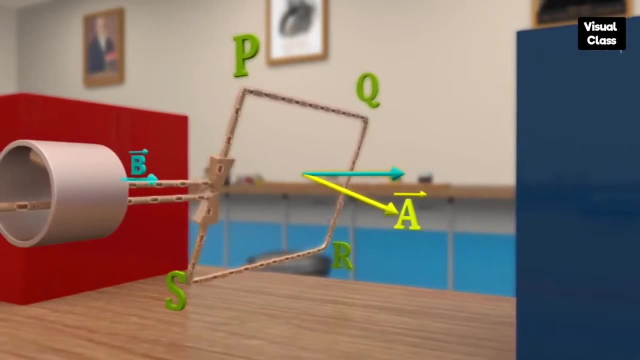 loop. Hence torque on the coil is equal to IBA sine theta. Let A bar be an area vector of magnitude of force. This gives the distance between the forces PN by PS. This gives the magnitude A normal to the loop. By curling fingers of right hand in the direction of thumb. 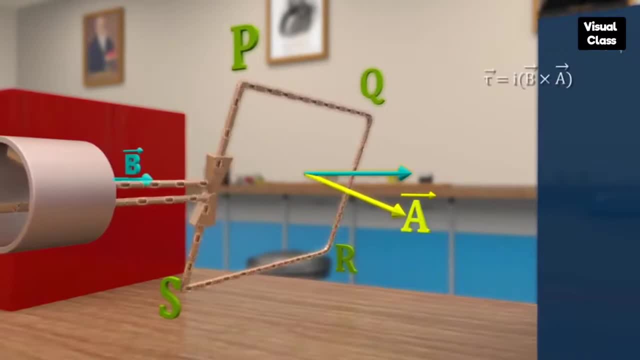 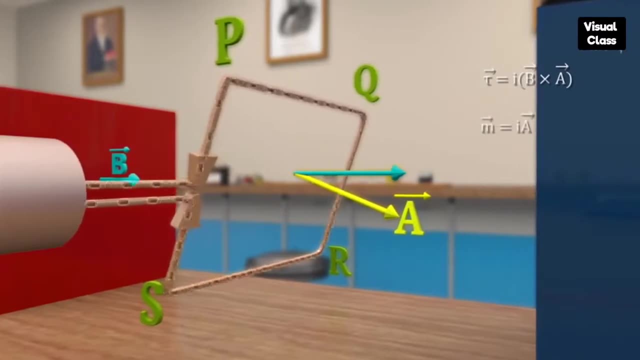 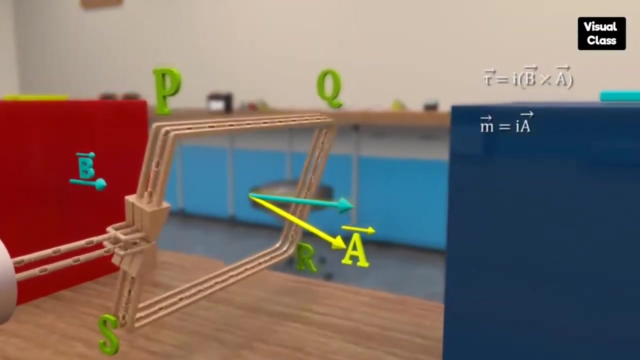 gives the direction of A bar. Net torque can be written as I A bar cross B bar. I A bar can be replaced with a vector called magnetic moment. Magnetic moment of a loop is the product of current and area vector. Torque on a loop is simply M bar cross B bar.